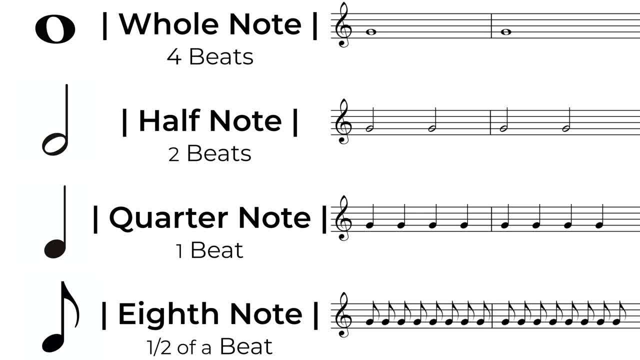 An eighth note is worth a half a beat of sound and fills up an eighth of the measure, giving us room to have eight eighth notes to equal a total of four beats in the whole measure. Individual eighth notes look like this, but we most commonly see them like this: 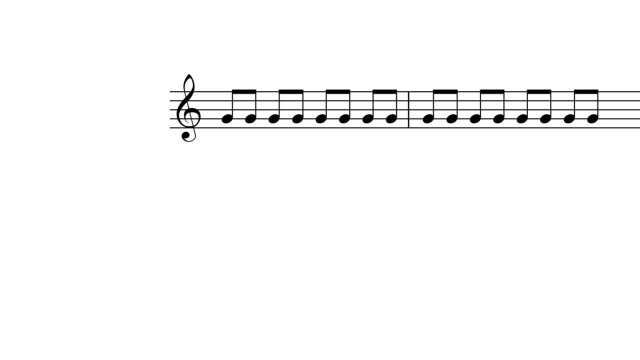 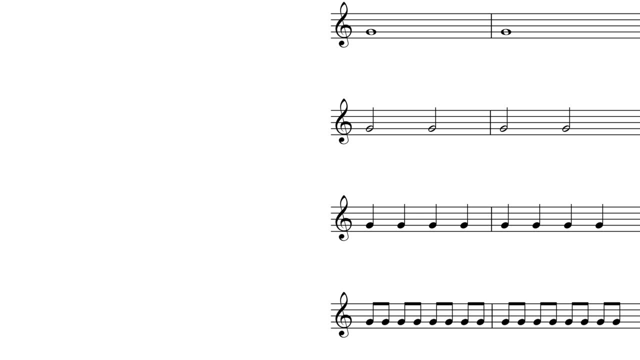 where they are grouped in pairs of two. This helps us visually to see where beats one, two, three and four are in the measure. A pattern we can notice here is how the rhythm values are essentially being cut in half each time. A whole note is divided equally into two half notes. 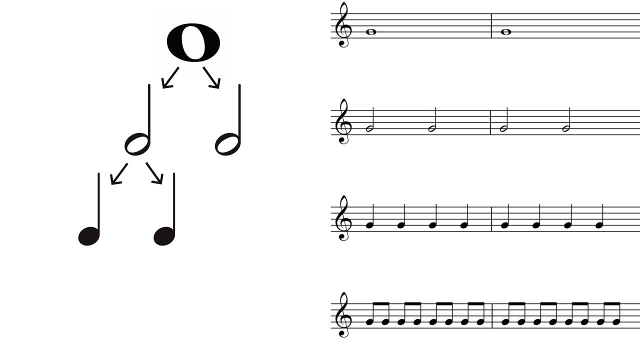 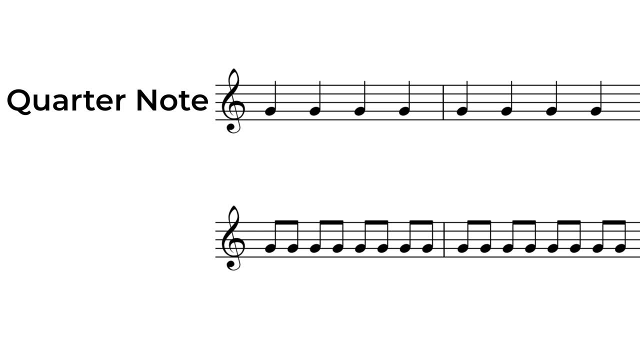 a half note is divided equally into two quarter notes and a quarter note is divided equally into two eighth notes. When quarter notes are played, they go exactly with the beat and are counted like this: one, two, three, four, Since eighth notes are worth a half a beat each. 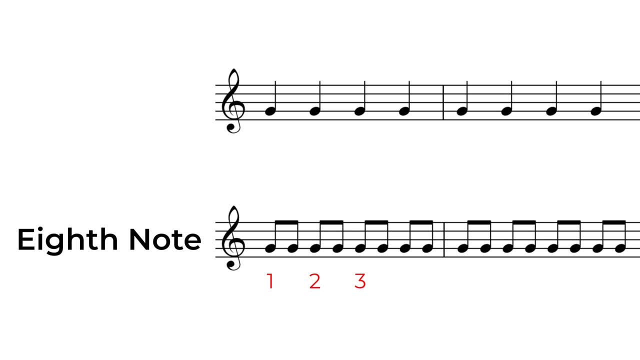 we need a way to count beats one, two, three and four, as well as the notes that happen in between. We do this by simply adding the word AND, in between, each number. So eighth notes are counted like this: one and two and three and four, and In the same way that we have our rhythms of sound. 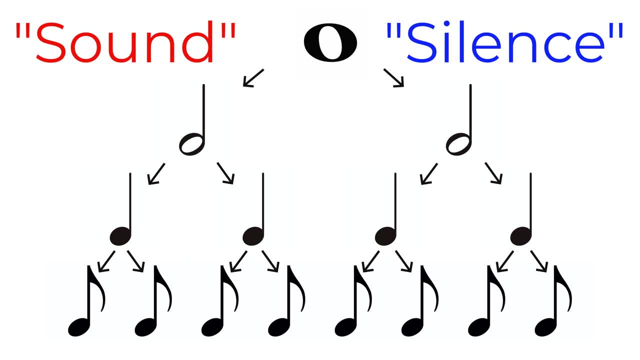 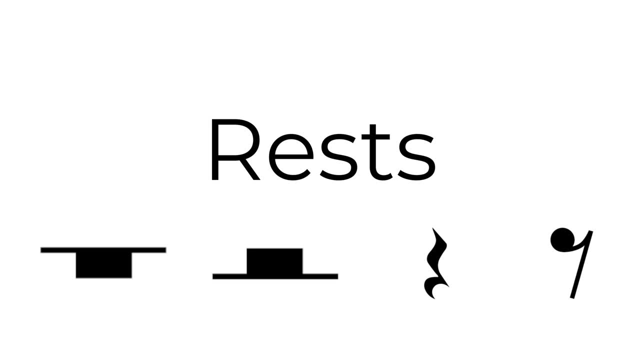 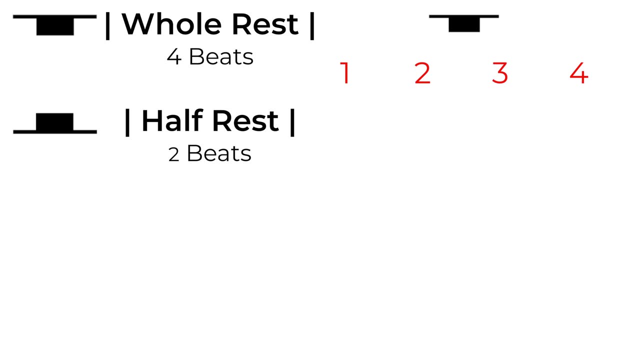 we also have our rhythms of silence. In music we call these rests, And rests, just like our rhythms of sound, are worth a certain number of beats. A whole rest is worth four beats of silence and fills up the entire measure. A half rest is worth two beats of silence and fills up half of the measure giving us. 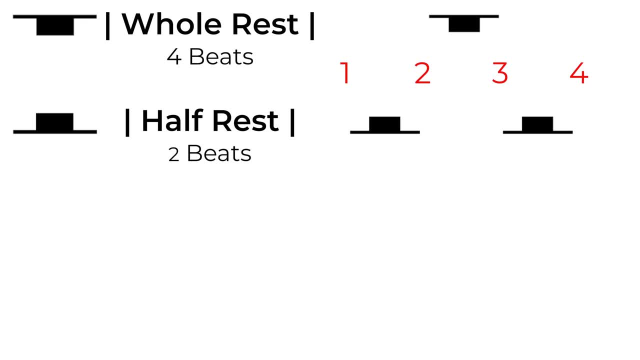 room to have two half rests to equal a total of four beats in the whole measure. A quarter rest is worth one beat of silence and fills up a quarter of the measure, giving us room to have four quarter rests to equal a total of four beats in the whole measure. 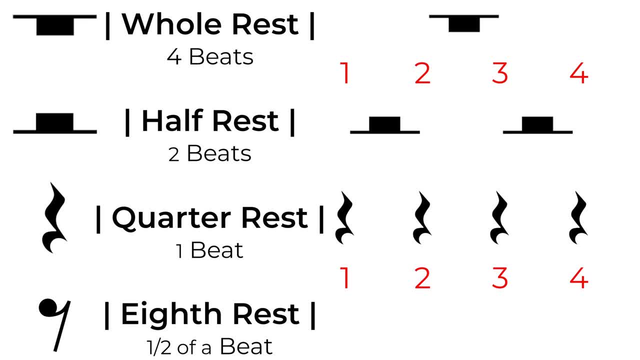 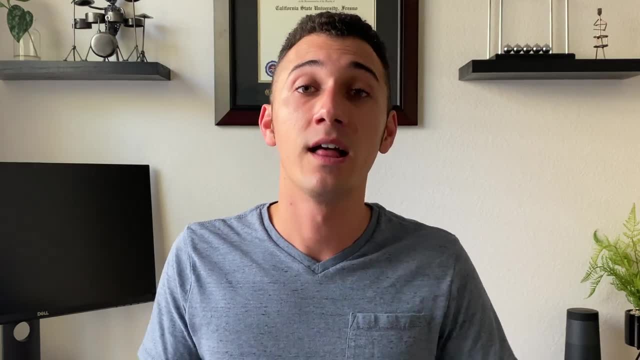 And an eighth rest is worth a half a beat of silence and fills up an eighth of the measure, giving us room to have eight eighth rests to equal a total of four beats in the whole measure. An important thing to note is that even when we have rests or silence, the beat continues to move.